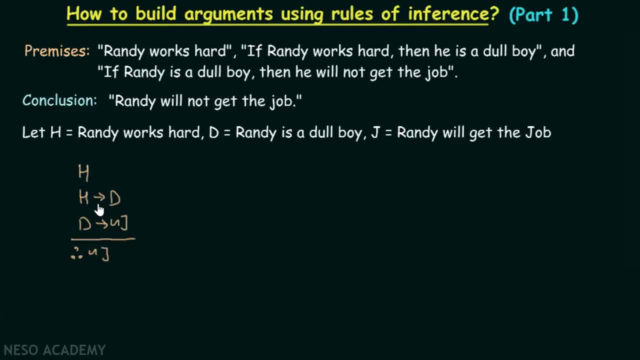 we need to come up with some conclusion by using rule of inference. Okay, like, for example: we can take H and H implies D, H and H implies D. Now we can apply the rule of modus ponens here and we can come. 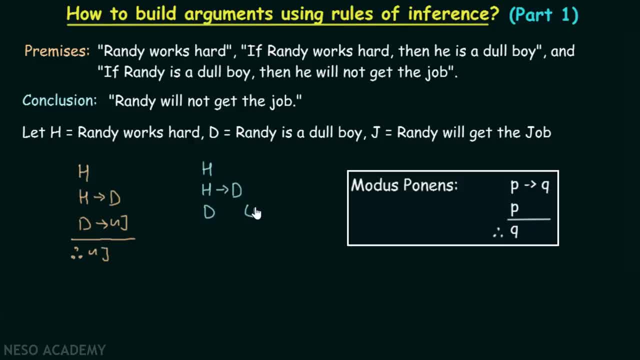 to this conclusion called D. Right, here we applied rule of modus ponens. Okay, so conclusion D can be obtained from these two premises very easily by using rule of modus ponens, And the next step would be to take another two premises. 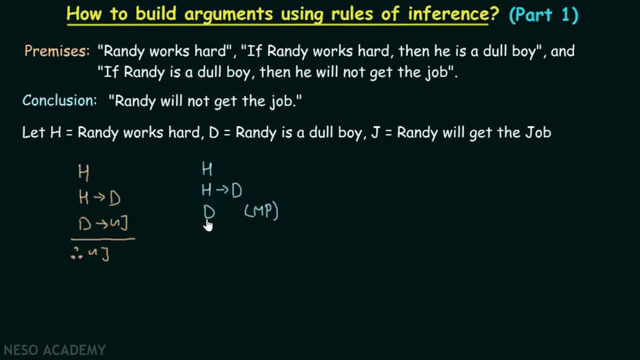 and try to come up with another conclusion. We can take D, and D implies not J, D implies not J. Please note down that it is not necessary that you would always have to take two premises from this place only. It is also possible that 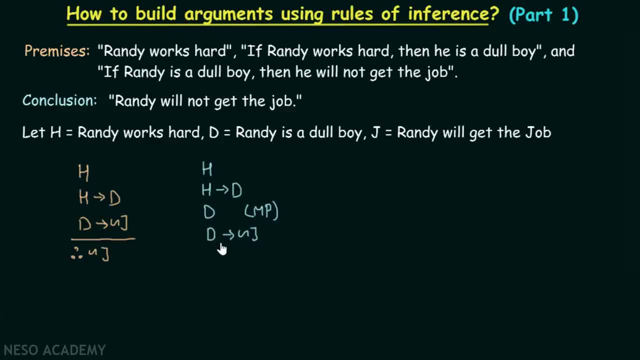 you can take conclusion of one argument as a premise to the other argument, Like in this case. we chose D, which is the conclusion of this argument, as a premise of this particular argument, As here also in case of D, and D implies not J. 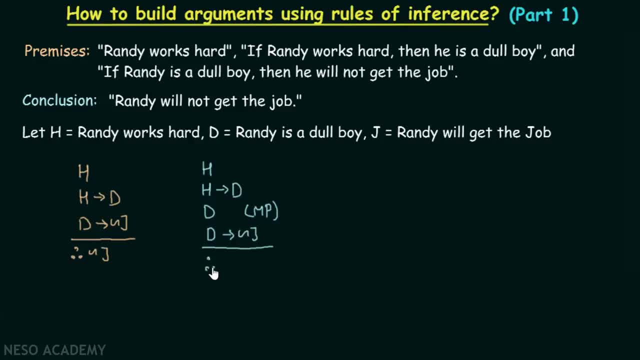 we can again apply rule of modus ponens to come to this conclusion, called not J. By again using the rules of modus ponens, Not J, is our desired conclusion right, That is what we want. So we can say that by using rules of inference. 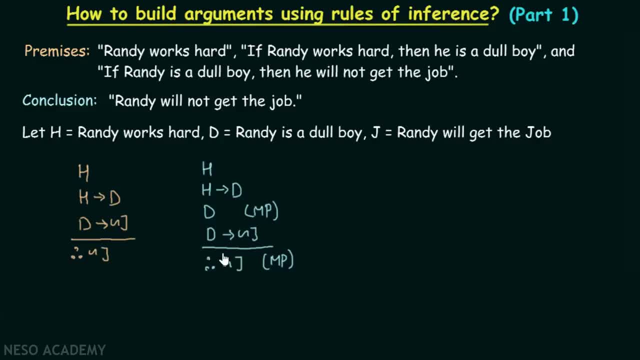 we can build this argument and finally we come to our desired conclusion. that is not J, And this is what we have to learn Now. it is also not necessary to take two premises at a time. In the worst case, you may take one premise also and you can apply. 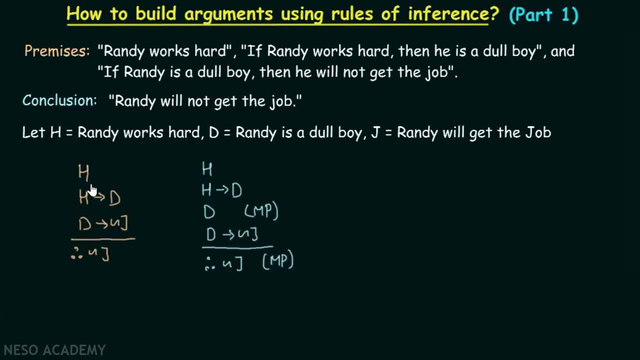 either simplification rule or you can apply addition rule. Right, But please remember, try to take two premises at a time and try to come up with some conclusion and go step by step. then It is also possible that the conclusion that you get from one argument 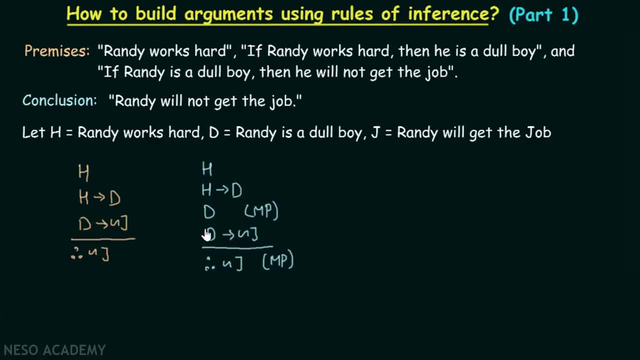 is of no use for the other argument. So it is not always the case that whatever the conclusion you are getting from one argument can be used as a premise for the other argument, And it may also be the case that conclusion of one argument can be chosen.